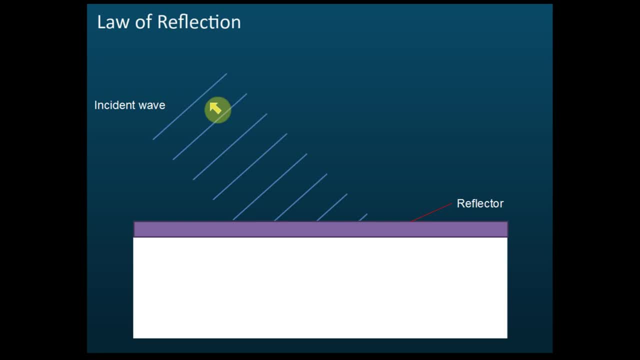 in this chapter is different from the diagram. in light Light we use straight lines to represent light, We use straight lines. We say this is light, This is called a light ray. But in this chapter we discuss wave, So we use wavefront. 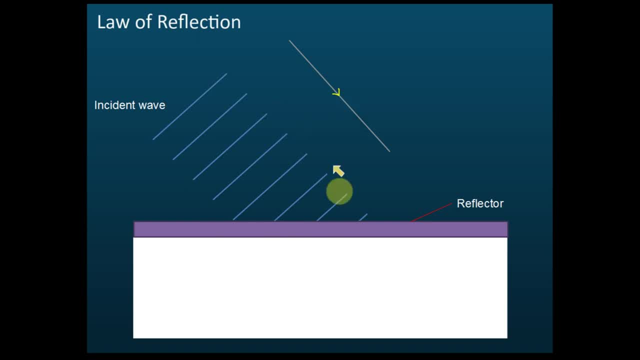 Wavefront. So it's different. This is light ray. This is wavefront. It's different. So we have incident wave. This represents the wave. This is a wavefront diagram. And then the wave hits the reflector. It hits the reflector, then it's reflected. Something wrong here. 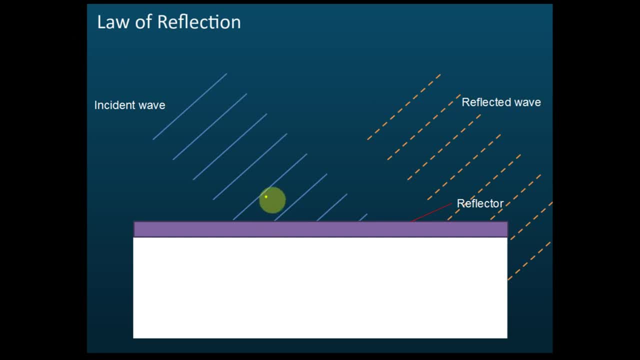 The reflected wave should look something like this. Something wrong here? Okay, The reflected ray here, So we'll learn how to draw this later. This wave, it hit the reflector and then this is reflected back If we draw the light. 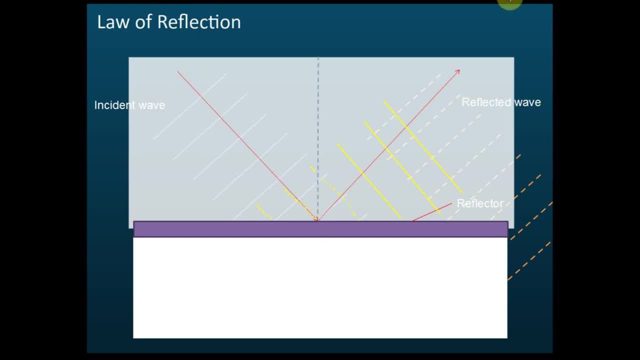 lines for the directions of the wave, and then we draw a normal at the center, then you will find that this is the angles of the incidence denoted by i and this is the angles of reflections denoted by r, and then, so these two angles, it should be the same. okay, these two angles should be the same. 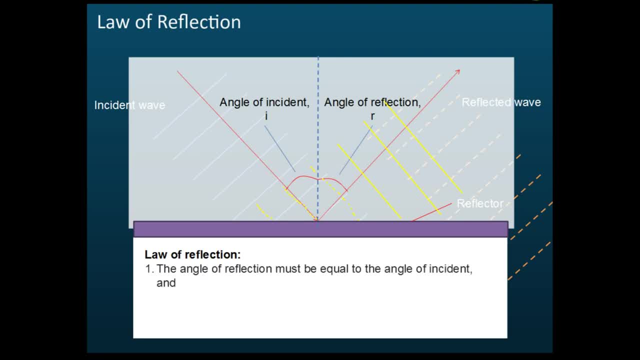 so that is the law of reflections. the angles of reflections must be equal to the angles of incidence. this is the first law. and then the second law. it says that the incident wave, the reflected wave and the normal. this is the incident wave, this is a reflected wave and the normal 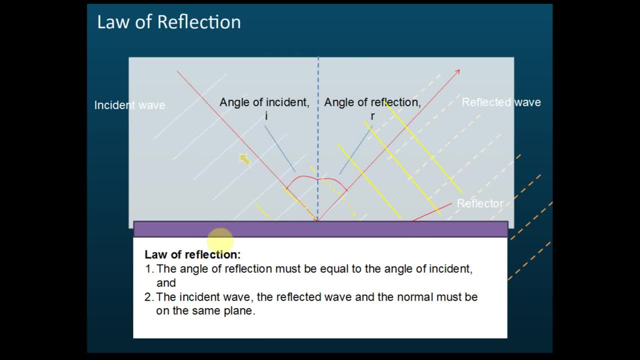 that must be on the same plane. same plane means same surface must be on the same surface. so this, these are the two laws of reflections, and you must remember this. you must remember or you must memorize. this must remember you because this can be asked in your uh structure questions or essay questions. the law of